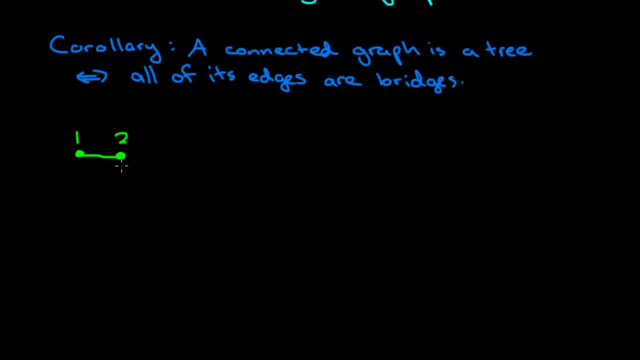 then there's a tree like this. Well, that's pretty simple. That's a tree on two vertices- Pretty boring. But if we have three vertices- one, two, three- I can see several different ways of making a tree, either like this or like this, or like this. 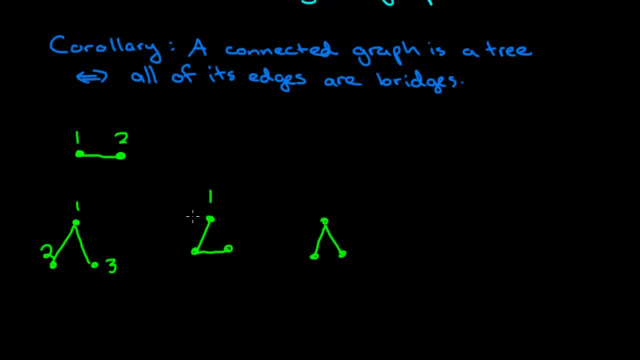 If this is one, two and three, this is one, two and three, But even though these are three different trees in terms of the labeling, these are really isomorphic. These are isomorphic. So there's two ideas here. 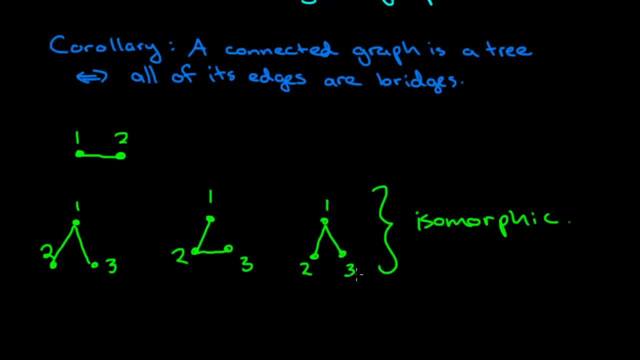 One idea is to figure out how many trees are there like this on a given set of vertices, and then the other idea is to think about which ones are actually truly distinct, Which ones are, Because I would call these all the same in terms of isomorphism. 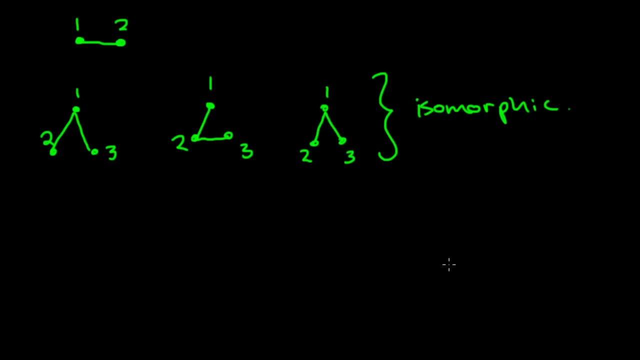 So in fact we know the answer to this question. So let's first look at the question of knowing the vertex set and seeing how many possible trees there are, And that's called Cayley's formula. It tells us that if we have a vertex set V of n elements. 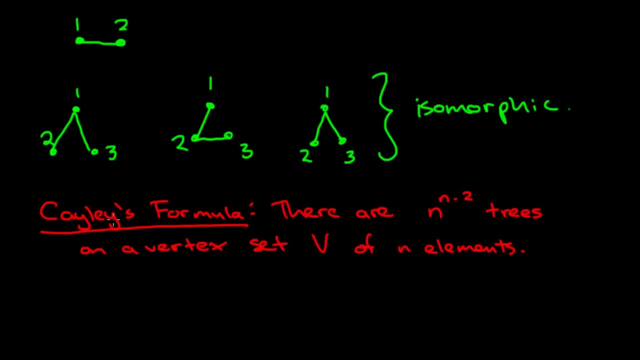 like in this case. we had one, two, three as the vertex set. then there are a total of n to the power of one minus two trees on that vertex set. So in this particular example we have n equals three and the total number of trees should be three to the power of three minus two. 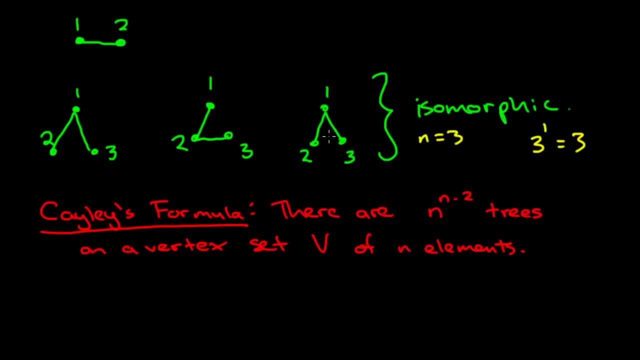 so three to the power of one gives three, And that's what we had here. So this tells us that there are certainly many, many, many trees on a given set of elements, but when we want to know how many trees are there in terms of isomorphism, 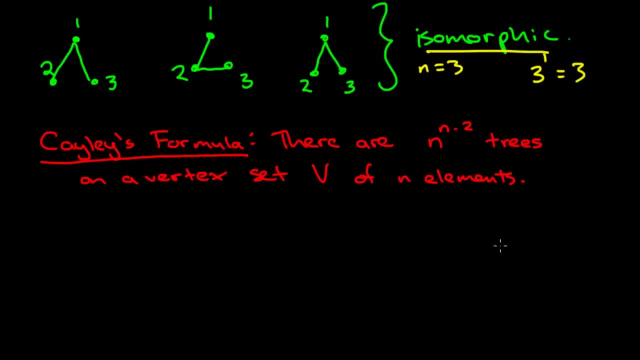 then we can take a look at this following table to give us a little bit of an idea. So, on only one vertex, we only have one non-isomorphic tree. It's just a single vertex without any edges, With two vertices. we have just the simple path on two vertices. 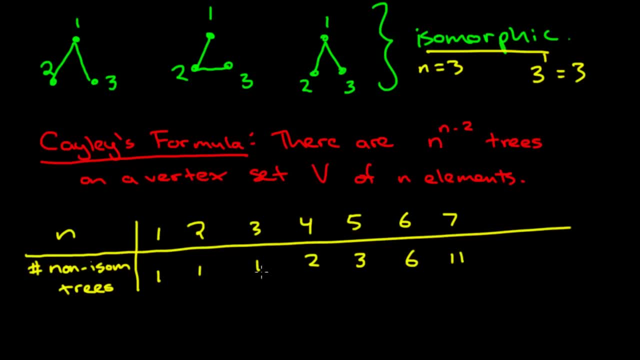 With three vertices. there's only one non-isomorphic tree on the three vertices. These are the three labeled trees on three vertices, but we saw that they're all isomorphic. They're all just a path of length two. So that gives us. 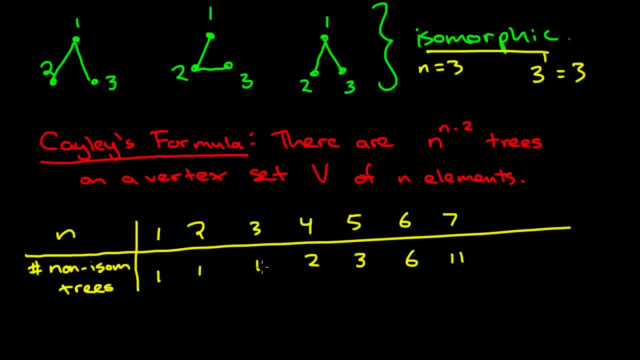 one non-isomorphic tree when we have three vertices, And it might be good as an exercise to try to find the two non-isomorphic trees of order four and find the three non-isomorphic trees of order five. Of order six. there are six non-isomorphic trees. 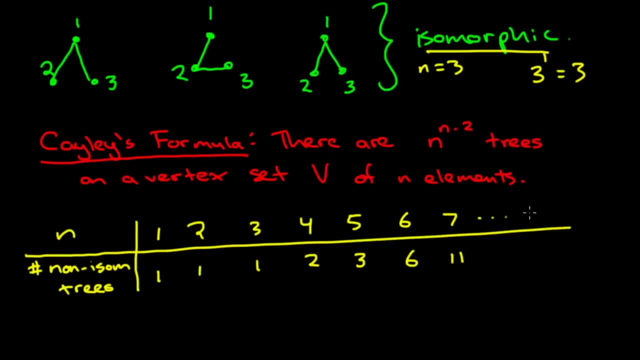 and in fact this number starts to grow quite a lot By the time we get to just 16 vertices, we already have 19,300.. So that's 120 non-isomorphic trees. So certainly we don't need to look for all of these right now. 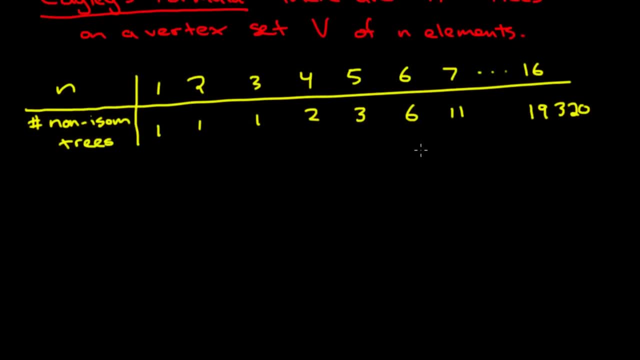 But what we could do is take a look right here. at this case, Let's take a look at the six non-isomorphic trees of order six and perhaps pause the video and see if you can find them, and then, when you play it again, you'll see the answer. 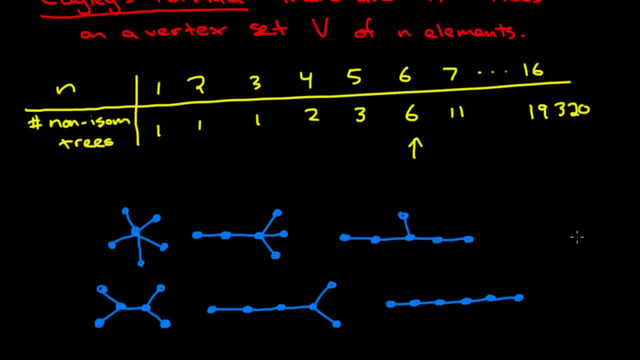 All right, so here they are. These are the six non-isomorphic trees of order six and, in fact, if you were to try to draw a connected graph on six vertices that has no cycle, you are going to get one of these six drawings. 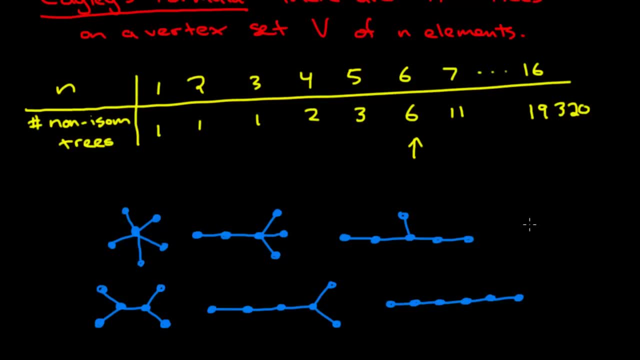 Of course your drawing may look slightly different, but upon inspection you'll find out that it's isomorphic to one of these six drawings. Now in a tree, we can see that some vertices have degree higher than one, but there's also several vertices. 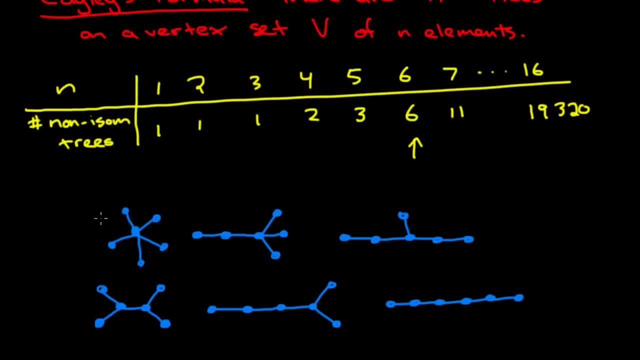 that have degree exactly one. So for example, in this graph, right here we have five vertices of degree one and here we have four vertices of degree one. here we only have three vertices of degree one and down here we only have two vertices of degree one. 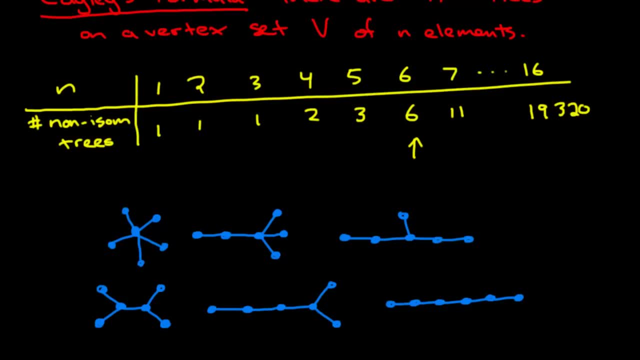 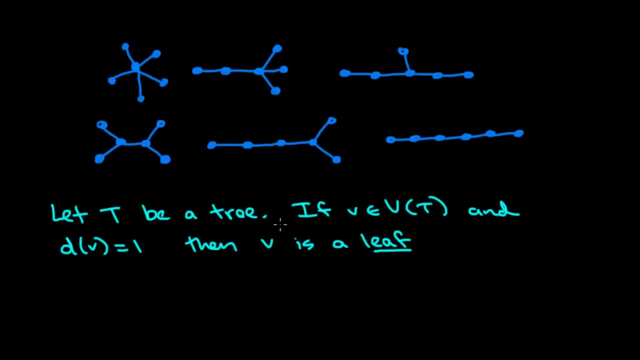 Now, in a tree, a vertex of degree one has a special name: It's called a leaf. So let's write this down: If T is a tree and we have a vertex in that tree which has degree one, then that vertex is called a leaf. 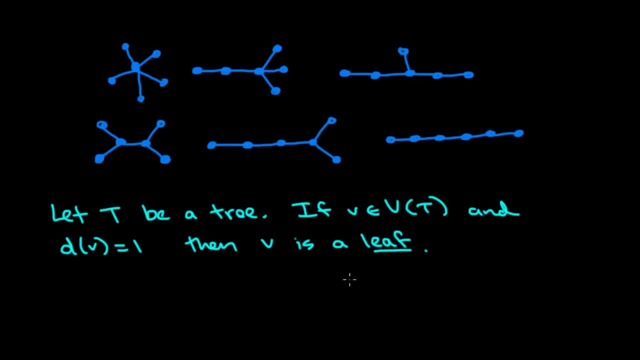 Now the first little corollary we have about- I'll just call this a fact, really about trees, is that every tree with at least two vertices has at least two leaves. Here it is, so we have any tree T and the number of vertices of that tree is at least two.